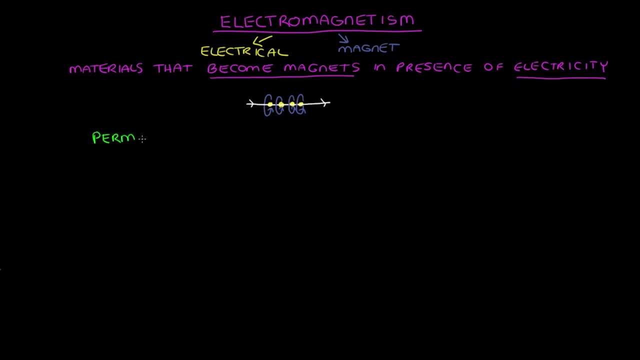 This makes electromagnets quite different from permanent magnets. So let's take a look at that and compare permanent magnets to electromagnets. Electromagnets are typically made of loops of wire in a coil. The wire is typically made of metal like copper and wrapped around pieces of metal like iron, nickel or cobalt. This is different. 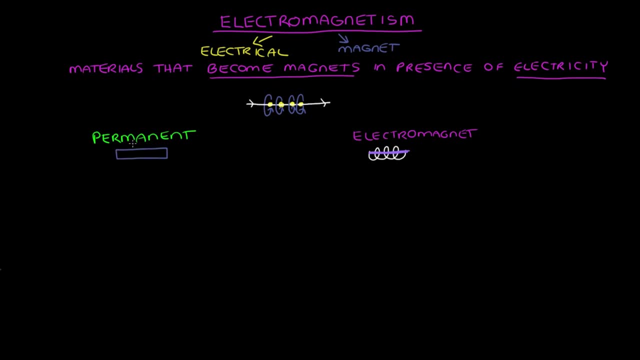 from a permanent magnet, because permanent magnets don't need this wire. Permanent magnets also have fixed poles. You can't change the north and south poles on these magnets, But, as we now know for electromagnets, we can change these poles by changing the direction of the electrical current. 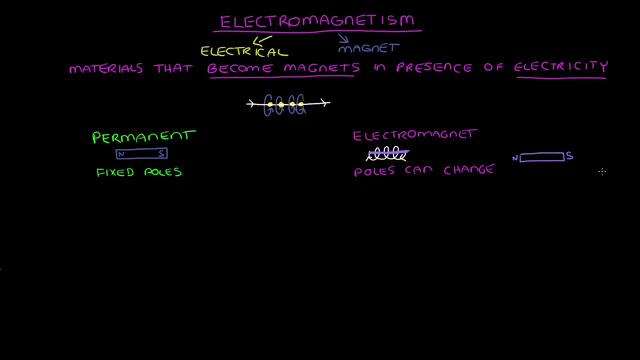 So if we have an electromagnet with a north and south pole that looks like this and a current flowing in this direction, well, we can change the poles and the direction of the current. Permanent magnets have a fixed strength. But we just talked about how we can. 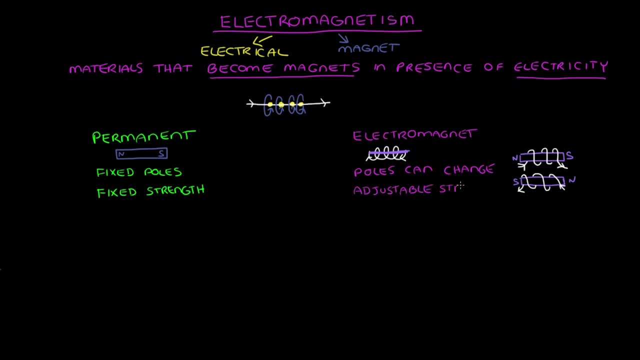 change the strength of electromagnets, so electromagnets have adjustable strength. And finally, electromagnets need a power source in order to generate the electricity required to produce magnetic fields. Permanent magnets do not need a power source, But this means that we can also turn electromagnets on and off. 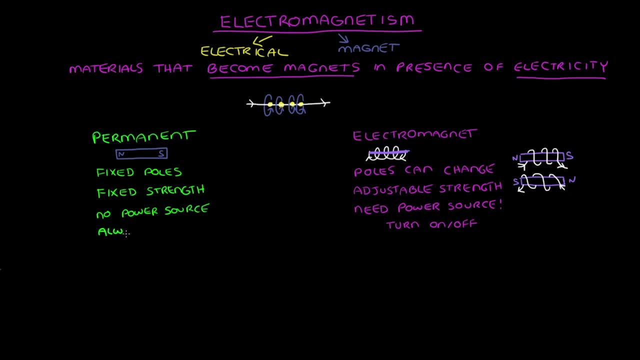 which is pretty cool when you think about it. On the other hand, permanent magnets are always on. Now you might be thinking: if electrical charge can affect magnetism, can magnetism affect electrical charge Absolutely? Let's look at how we can do that. The only way to do this is: 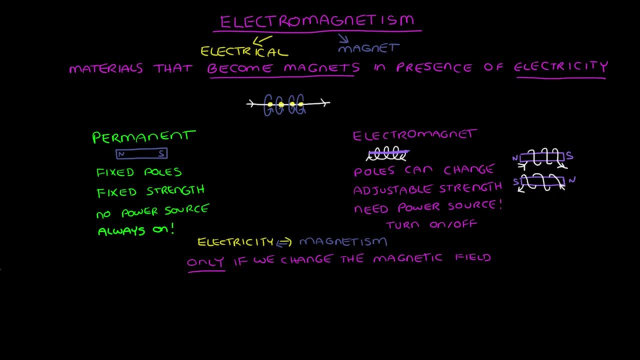 by changing the magnetic field around the charged particles. This can be done by moving magnets closer or further away from the particles, Or by spinning the magnets. In fact, spinning magnets is how most of the electricity we use in cities and homes is generated. A turbine spins a magnet. 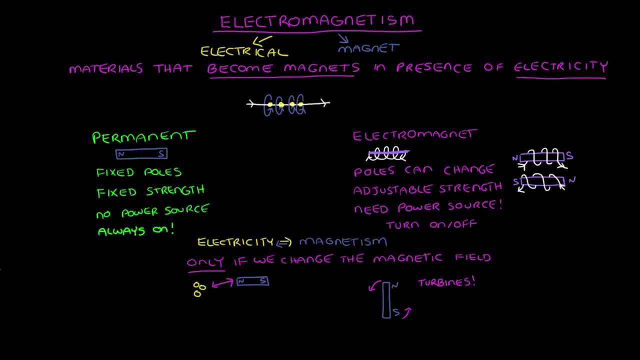 immediately inside a coil to produce electricity. And since electromagnets need a power source, this turbine is powered by wind. So you can see why electromagnetism is an incredibly important force, And this isn't the only important application of it.